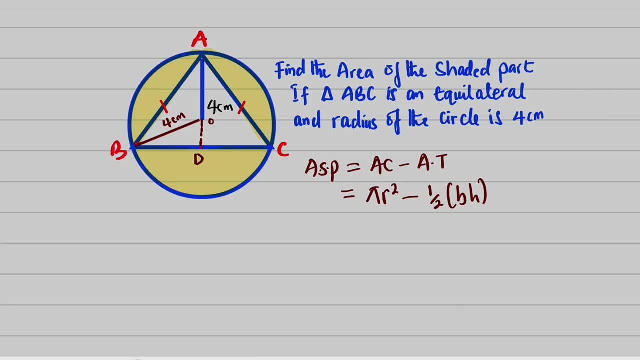 triangle has all its interior angles equal to 60 degrees, and you can see that this angle has just been bisected and therefore this one right here is going to be 30 degrees, This is going to be 60 degrees and this is angular 90 degrees. So therefore the height of this triangle, which is H, is equal to the 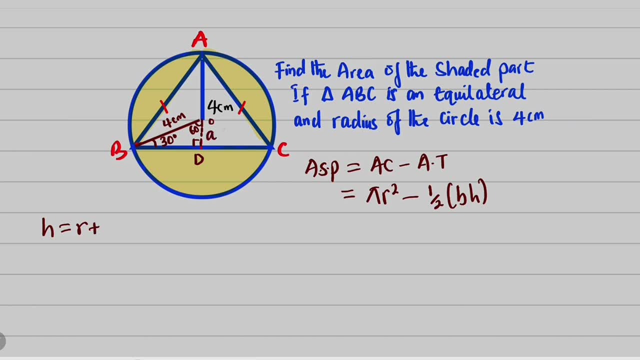 radius plus this point, let me call it A, which I have extended. So to find A, we can now multiply the radius by sine of that angle, 30 degrees, and this is equal to 4, which is the radius multiplied by 1 over 2, which is the same thing as sine. 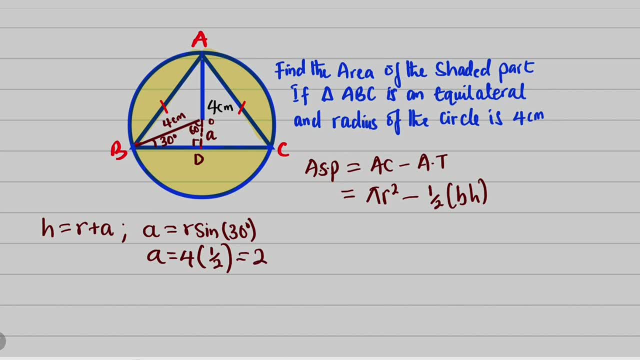 of 30 degrees, This is equal to 2.. So we can see that A is equal to 2.. We can now add it to our radius to find the height, and height is now equal to the radius, which is 4, plus A, which is 2, and this is equal to 6 centimeters. So now let us go. 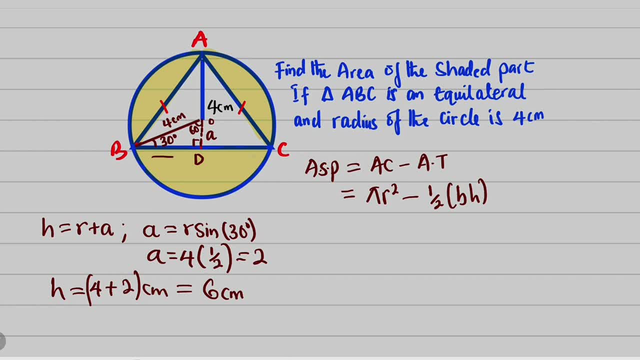 ahead and find the radius. So this is equal to 2 and this is equal to 6 centimeters. So now let us go ahead and find base. The base is this: line BD plus DC, But line BD and line DC are all the same. 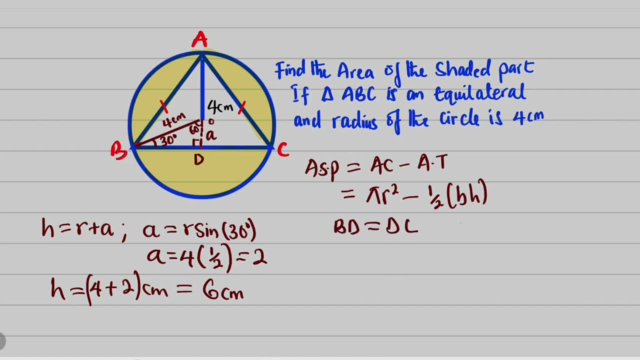 BD is equal to DC. Therefore, we can say that the base is equal to 2 multiplied by either DC or BD. But how can we find this BD? BD can be obtained by multiplying radius by cos of that angle- 30 degrees, And this is equal to 4. multiplied by cos of 30 degrees will be root 3. 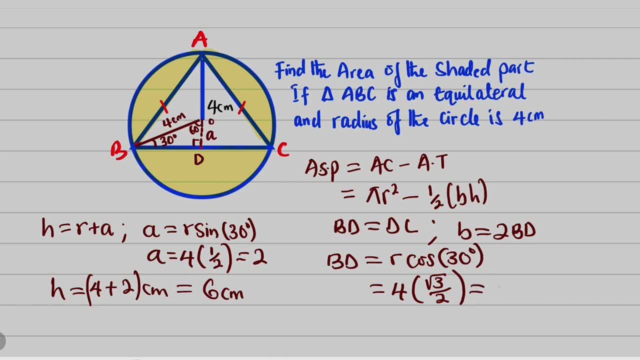 divided by 2.. And if you simplify this, you're going to obtain 2 root 3.. If line BD is equal to DC, then BD is equal to 4 multiplied by cos of that angle, 30 degrees, BD is 2 root 3. therefore, the base, which is 2 multiplied by BD, will now be equal to 2.